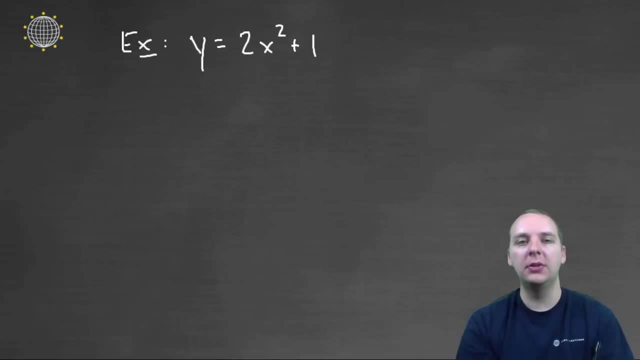 theory doesn't quite make perfect sense. let me show you with some examples. Here's an example of an equation written in rectangular form. It has X's and Y's, And let's see if we can parametrize this guy. So when we're done, we'll have X equal to something and Y equal to something. 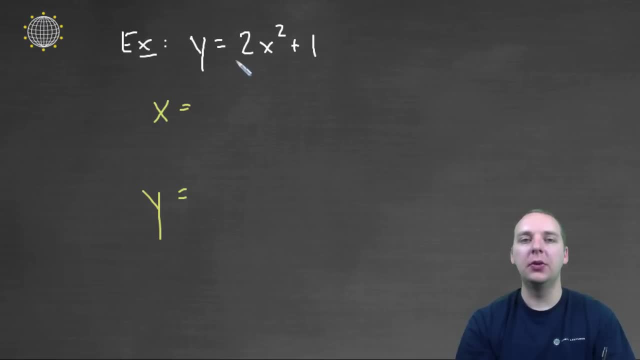 and I want this guy to be a parametrization of this equation here, And my tip earlier was: just always let the X just be T. And now we see why this works. It's because if we're given Y equals two, X squared plus one, but X is T, then you suddenly have Y equals two. 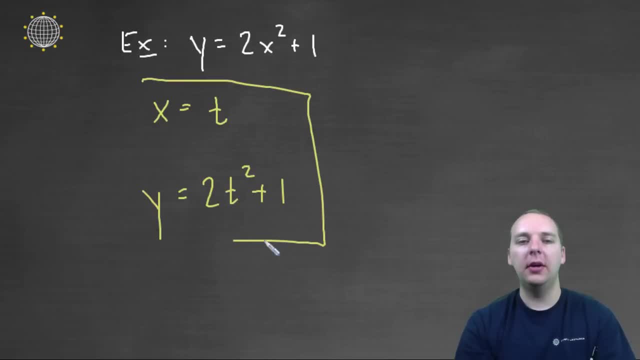 T squared plus one and you're done. There's nothing more to do. You've parametrized this curve here. This parametrization has an orientation that the original equation did not have, but the curves look the same And that's automatic. Usually if you have to parametrize something. 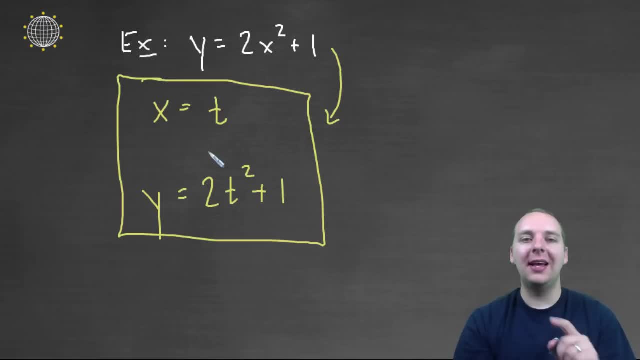 do that and you're done Now again. earlier I had said that's not the only way to parametrize a curve. let's look at some different parametrizations for this same problem, For this time. this time, let's let x equal. let's let it be 2t instead of just a t. 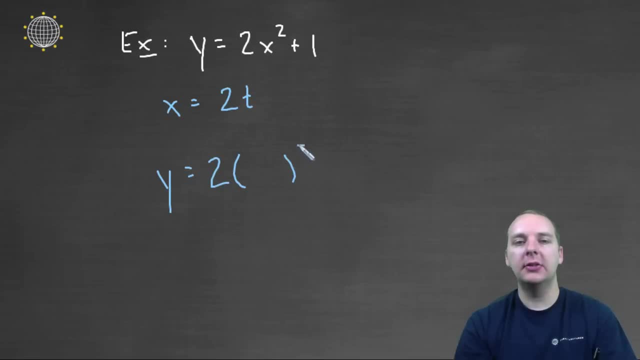 Well then your y, that used to be 2x squared plus 1,. we're just going to come back up here and we'll take whatever x was parametrized to be, in this case 2t. we'll substitute that value in for x, in this case 2t, and then we'll see how everything plays out. 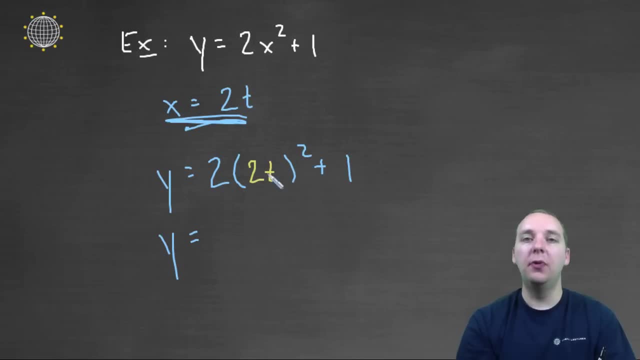 In this case y would be. let's see: 2t squared is 4t squared, and 4 times 2 makes 8t squared plus 1.. So if x equals 2t and y equals 8t squared plus 1, that's a different parametrization. 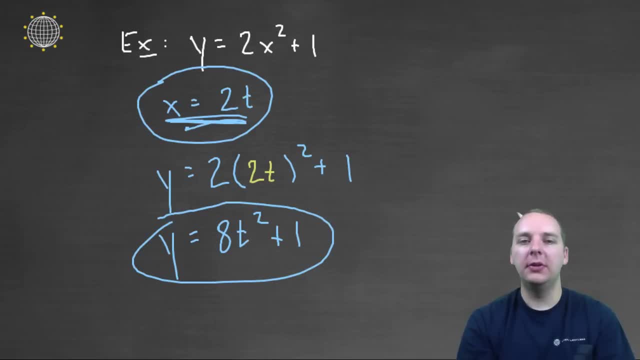 for the same equation. Now, what would be the practical difference between this parametrization versus this one? Well, I kind of explained this one in an earlier video. This one might sketch out the curve faster or slower than this parametrization does. 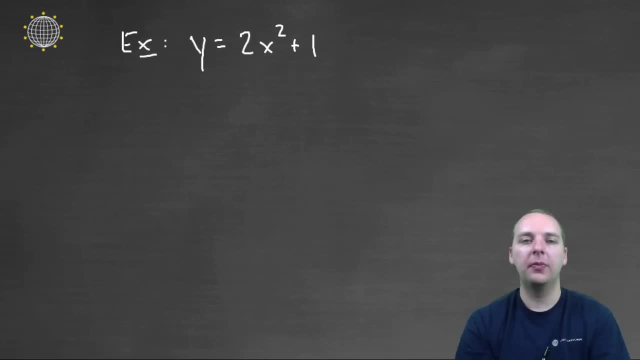 But it's still going to generate the same looking curve. Alright, let's do a couple more. How about this one? What if we let x equal, maybe this time t plus 3.. Well, in this case you'd have 2x squared plus 1, but in this case x is t plus 3.. 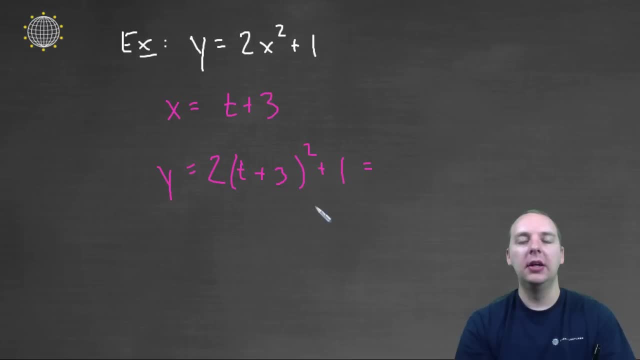 And so if you foiled that and simplified and all those good things, you would get y equals 2t squared, and I'll spare you the algebra. let's see plus 12t. let's see plus 19, I believe, if I did my algebra correctly. 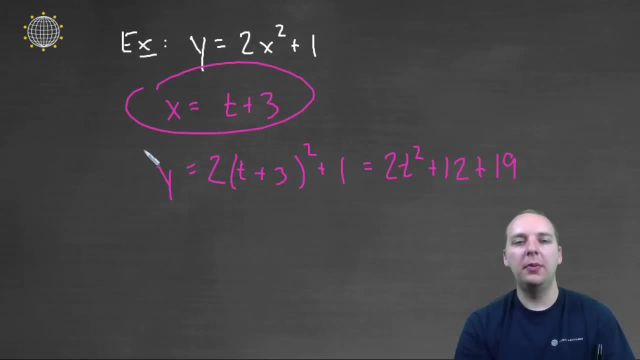 And you can check my math on that. But here we have a parametrization that's different than the first two. Ok, now the last one we're going to do is has a different spin to it. Let me do this parametrization and then we'll talk about how this one's different. 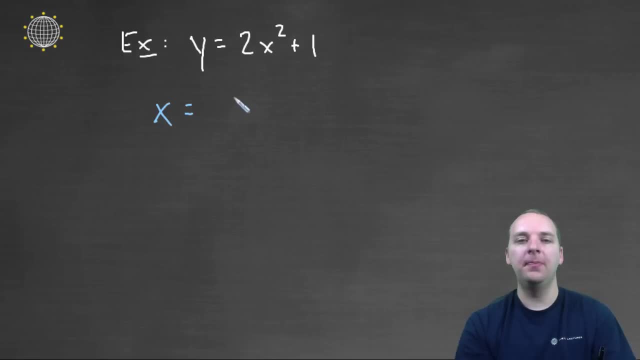 This time, rather than let x equal t, let's let x equal negative t. Then your y would equal 2 times negative t squared plus 1. Which would be 2t squared plus 1.. Alright, so let's think about this one for a minute. 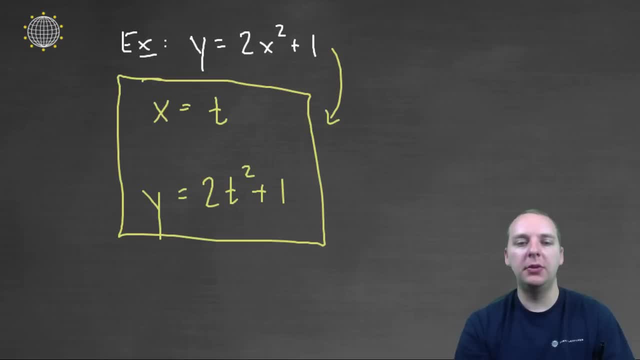 And actually let me go back to the very first parametrization I did. first This graph: y equals 2x squared plus 1 is a parabola that looks something roughly like this And you notice, based off of this parametrization, as t gets larger, x gets larger. 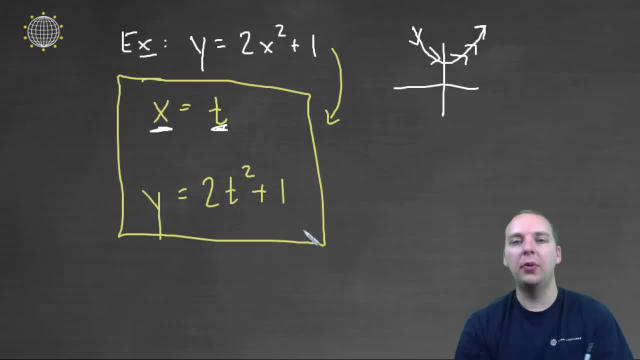 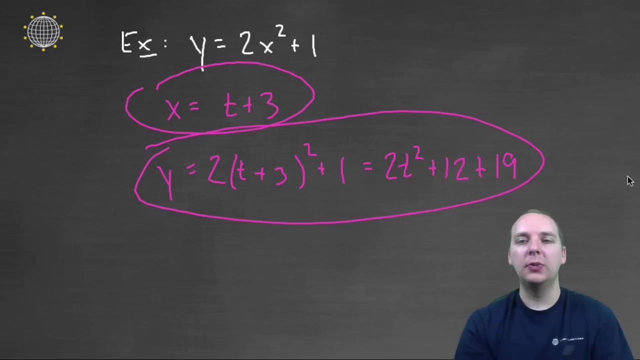 So the orientation would be in this direction. We would have orientation from left to right. Now for the second and third examples. you would have the same basic shape, but this one would progress through the curve faster or slower, as would this one. But the last one's a little bit of a different animal. 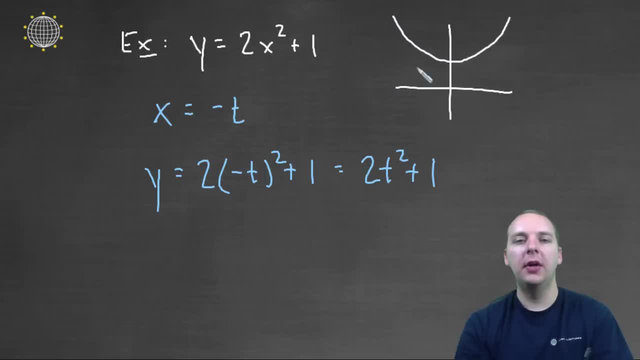 You would still have the same basic shape to the curve. but notice now: as the t gets bigger, the x gets smaller. Right, Because if t is 0, x is 0. When t is 1, x is negative 1.. When t is 2, x is negative 2..